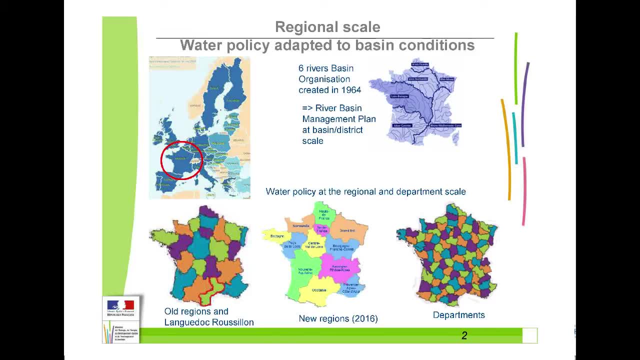 has its own water policy. Each river has its own water policy. Each river has its own water policy. So we have a plan for each river basin. Each district will have so the elaboration of River Basin Management Plan. So Languedoc-Roussillon is located here on this map. I do not know if you see the pointer. 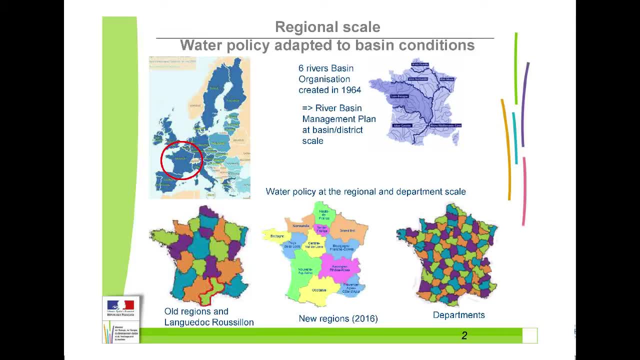 So it is a so we had a new region in 2016.. So now we are in Occitania region, And Languedoc-Roussillon is this part of the new West facing location region, and it is mainly in the district of Rhone-Méditerranée. So we have to work at. 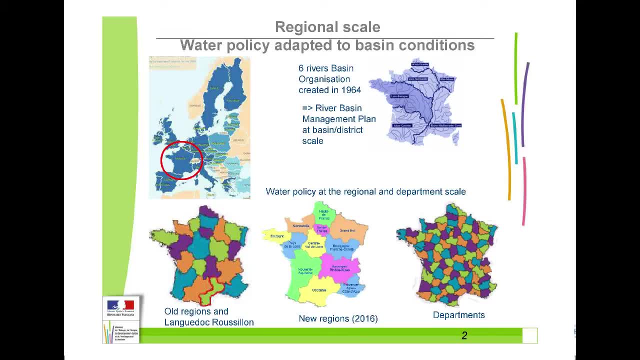 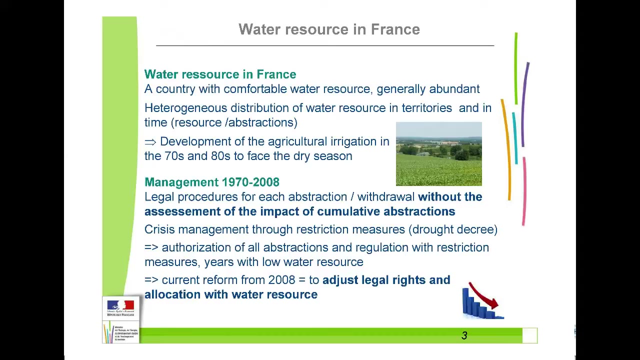 different scale. we are working partnership with department services, So let me give you some overview of historical water management in France. and so, first of all, we could say that France is a country with comfortable water resource, but we have a dry season and generally between June or July until September and October. That's why. 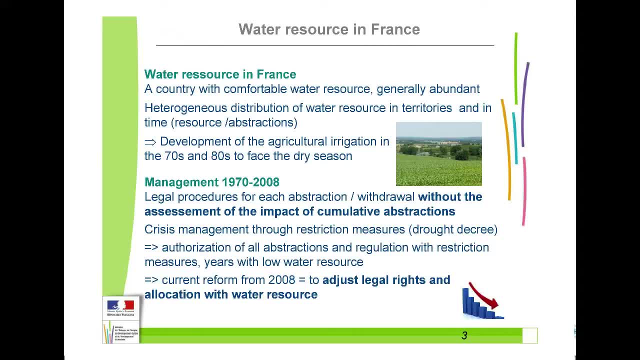 we have to develop agriculture irrigation in the 70s and the 80s to face the dry season, And so how was done the map management between the 70s and 2008.. It was done through a legal procedure for each abstraction. 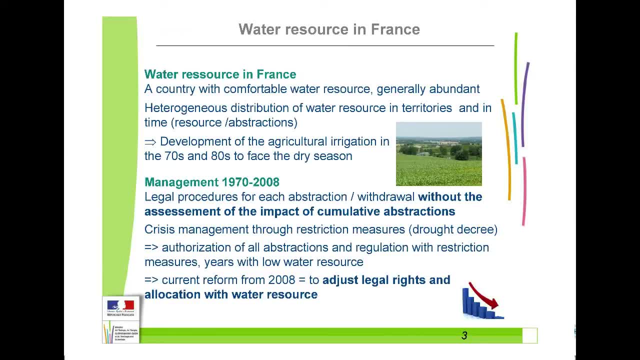 but there wasn't any assessment of the impact of cumulative abstraction. So it was scheduled to make a regulation through the crisis management, through restriction measures. But the thing is that we had more and more to use crisis management, so it was not possible. That's why we had the current reform from 2008, with the objective to adjust legal rights and allocation. 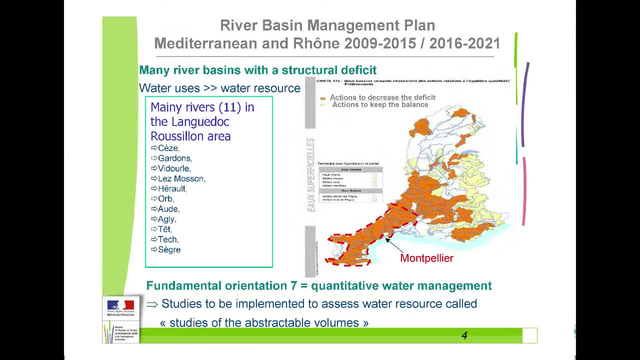 to water resources. In this map you can see this is a map of the river basin management. This is the management plan of the district Mediterranean and Rhône, That is to say that it includes Rhône River, all the affluents and all the Mediterranean rivers. 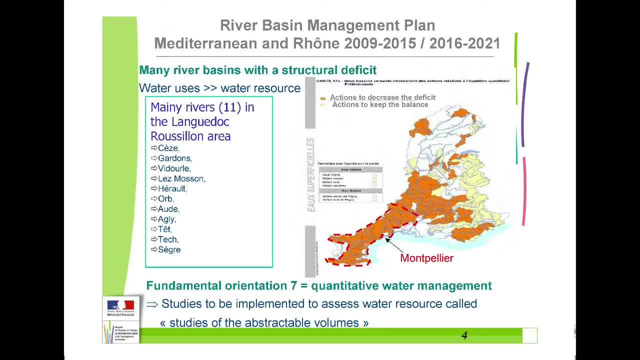 You can see that Montpellier is here. we are in the Languedoc-Roussillon area And on this map, the river basin, which were considered in 2009 in structural deficit, were closed. They were not in a range. 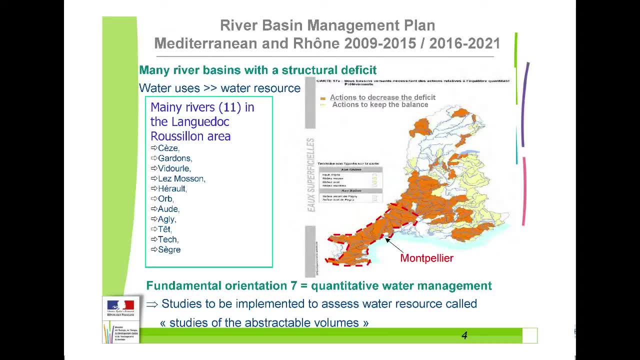 That means that in this river basin we have to implement action to decrease the deficit. So you can see that in Languedoc-Roussillon we have plenty of rivers that are concerned, exactly 11.. In this presentation I won't speak about specific aquifer management, because we have the same case. 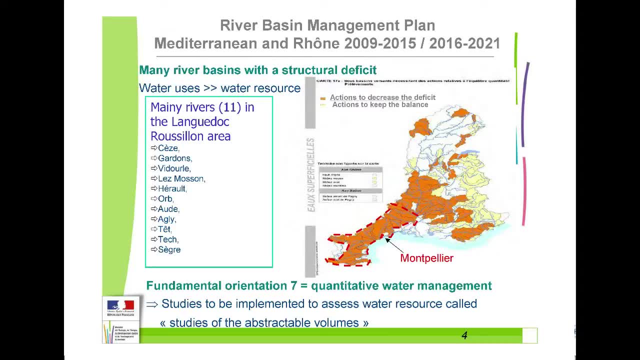 the same management for several rivers. We have several aquifers, so groundwater, that are not directly linked with rivers and surface water bodies. So we have in this RBNP several fundamental orientations and the seven is dedicated to quantitative water management. So this fundamental orientation asks us to implement a water management plan. 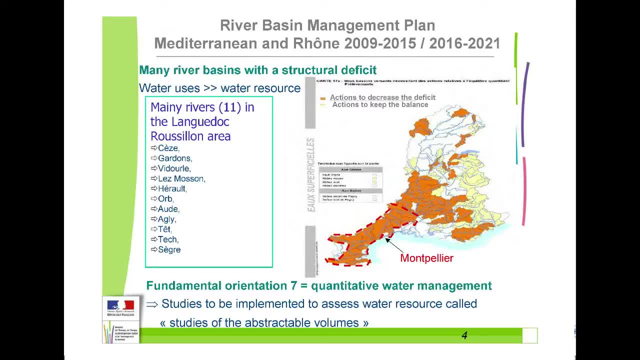 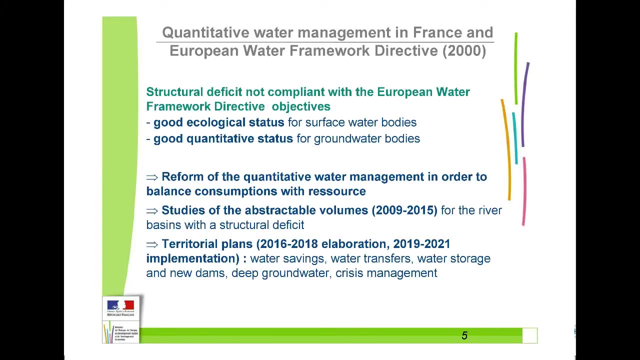 It asks us to implement studies to assess water resource and we call these studies studies of abstractable volumes. Of course we have to be compliant with the water from our directive and its objective that are to reach good ecological status for surface water bodies and good quantitative. 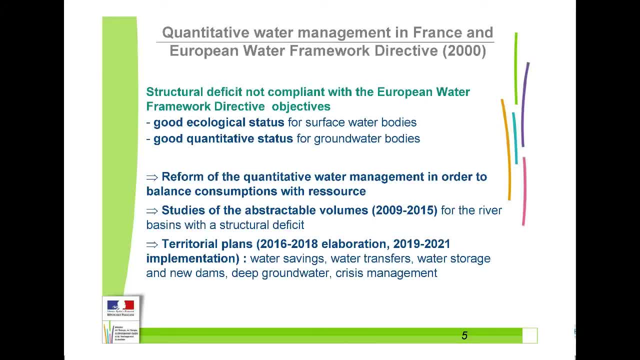 status for groundwater bodies. So we have to implement this waveform in order to recover the balance, And so we had to implement the studies of abstractable volumes between 2009 and 2015.. And then it was scheduled to first elaborate territorial plans, then to implement these. 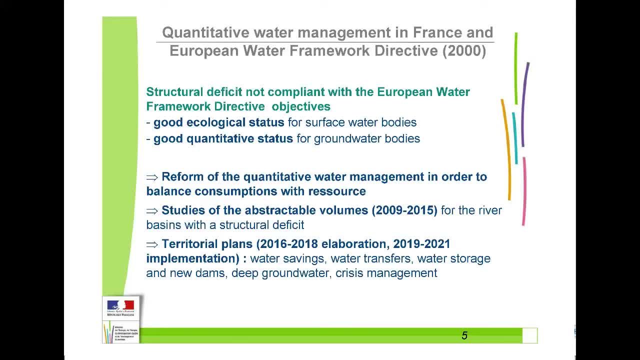 plans. these territorial plans between 2019 and 2021.. To say that we are in the cycle of the RBNP- the current RBNP from 2016 to 2021. And these territorial plans includes different actions as water saving, so that's an important. 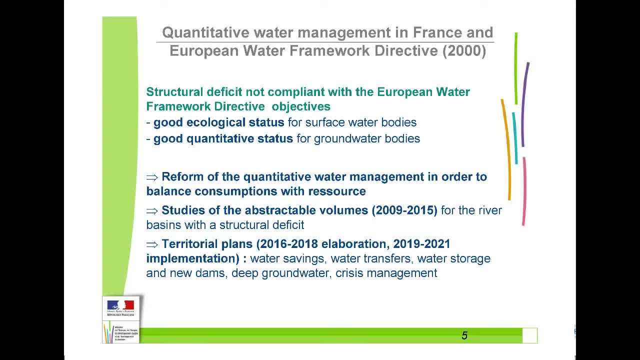 action. Then water transfers from river basin or groundwater resource. who are not in structural deficit as well? So one river, so a lot of region. a lot of territorial plants want to use this resource, but we have also now to manage this resource. 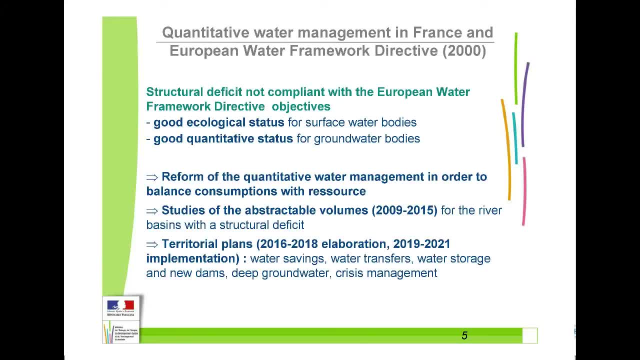 And then we have also water storage in Ulam, because you will see that we have to face dry season, where we have natural flows that are low and, moreover, abstraction and demand are very big. So that's why it's important, So that's why it's an interesting solution to store water in the humid season either. 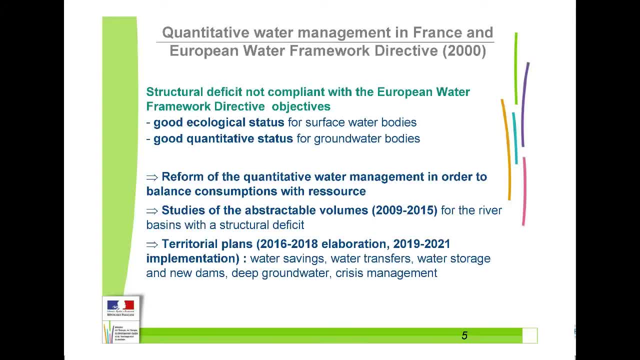 in dam or in some groundwater and to use that in the dry season. We have also deep groundwater management in this plan. that can be a solution and crisis management, But in the strategy we do not. we want to adapt the abstraction in order to use crisis. 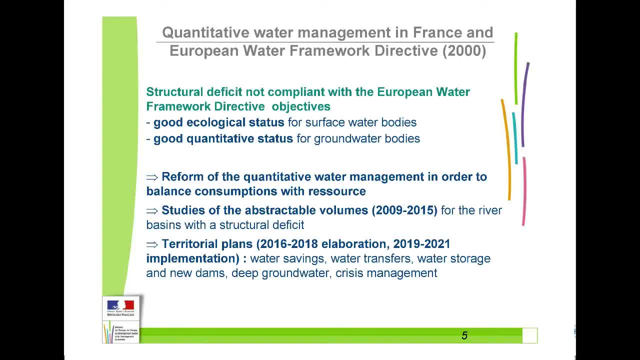 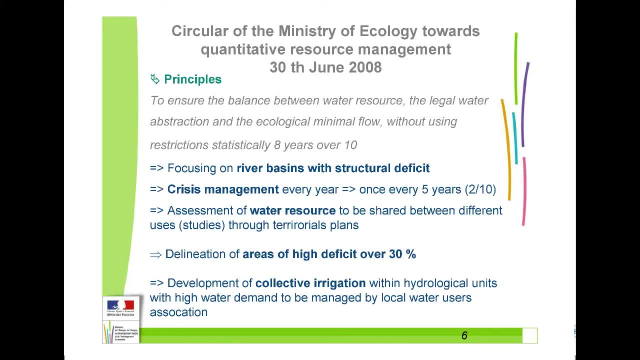 management In order to use crisis management only. you will see two years over ten years, or only one year over five years. So that's the principle of the French circular of the Ministry of Ecology towards reconstructive resource management. So the principles are to ensure the balance between water resource, legal water, abstraction. 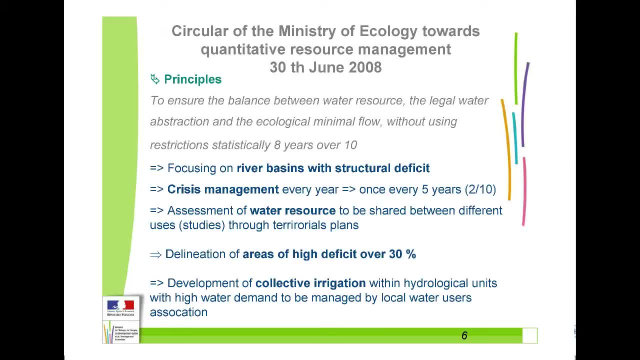 and ecological minimal flow, But we do not have to use restriction and so crisis management more than two years over ten. So the work is focusing on river basin with structural deficit. We have to access water resource to be shared between the different uses and through territorial 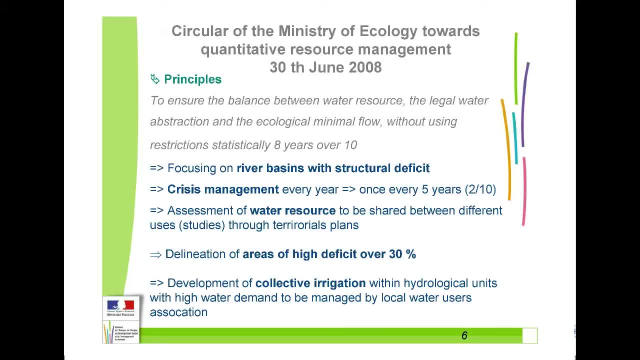 plans And there is also the action of delineation areas of high deficit, around 30 percent of reduction of the current abstraction And another solution, another action is to make to use the collective irrigation within hydrological units with high water demand and to be managed by local water users as 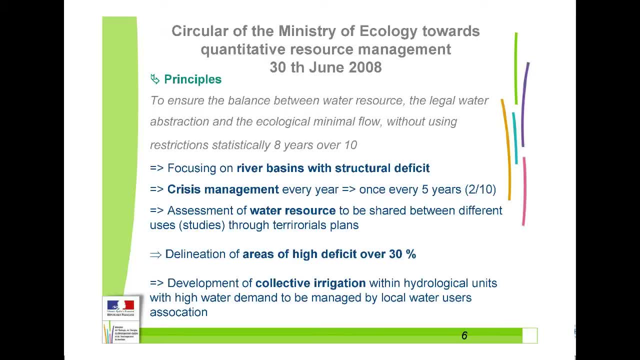 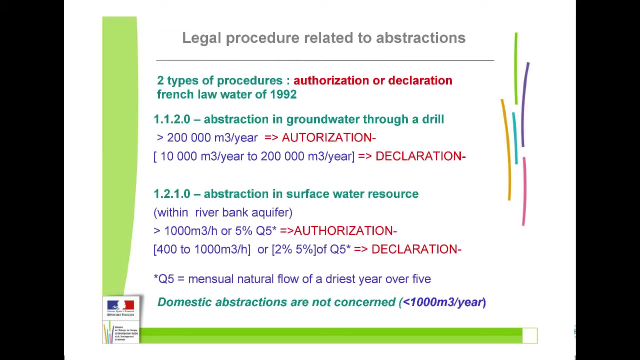 a session. That means that administration cannot all manage if we have got plenty of users and of water, So we have to use the collective irrigation. We hope that it will work better through a unique actor managing this collective irrigation. So then we have to implement this reform. 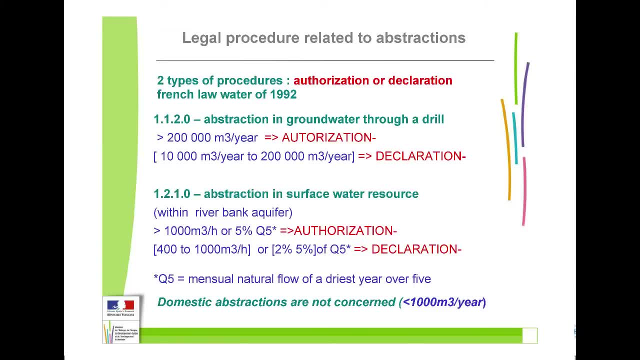 We have some legal tools that I will present to you quickly. So we have some tools for general case. First I will show you the legal tools. I have to precise that domestic abstraction are not concerned when the abstraction is less than 1,000 cubic a year. 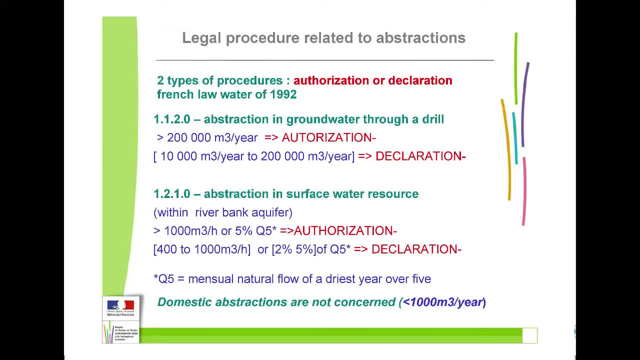 And then either we have got one for abstraction in groundwater not linked with surface bodies and another one linked to abstraction in surface water resource. So, depending on the level of abstraction, We are either in the procedure of authorization or declaration. so declaration is simpler. 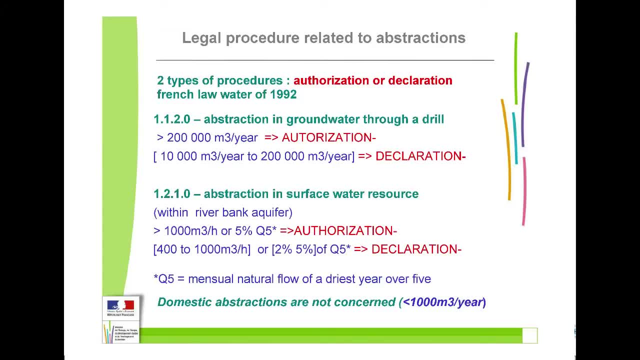 So these tools came from the French Low Water of 1992.. You can see that here that is the impact, and to identify the kind of procedure- either authorization or declaration- We are using the Q-SAN, What we call Q-SAN. 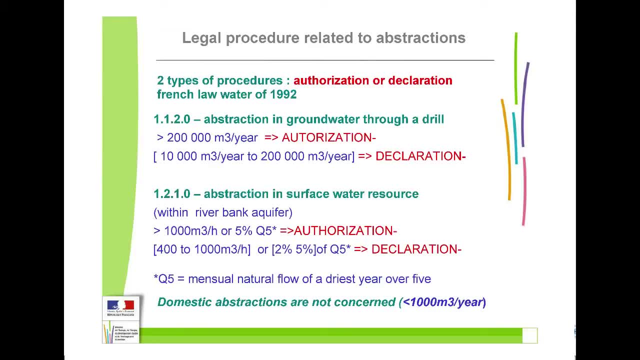 Q-SAN, Q-SAN, The National Natural Flow of the Dryers Here, Over Five So. but this thing is that it doesn't take, it doesn't make the assessment of the cumulative impact of all the abstraction, And that's what we will try to do in the current territory at that. 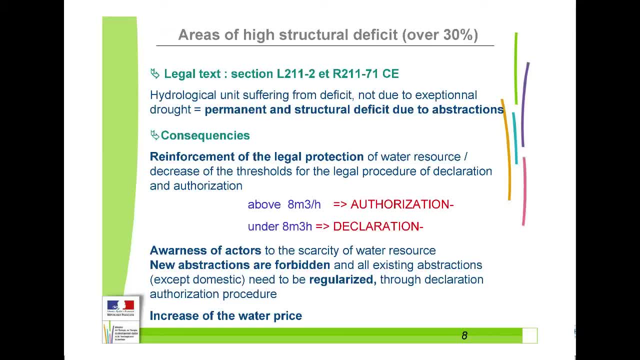 In the case of high structural deficit, we have another tool. So first definition of this, This is the Q-SAN, this area. so there are hydrological units suffering from this deficit that it's not due to exceptional droughts. 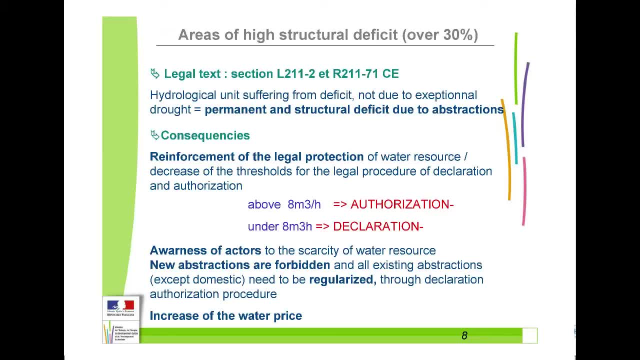 That's to say that abstractions are very too high. So the consequences are that we can reinforce the legal protection of this water resource and decrease the threshold. so it allows also the awareness of archers to scarcity of water, so it can improve the behavior. 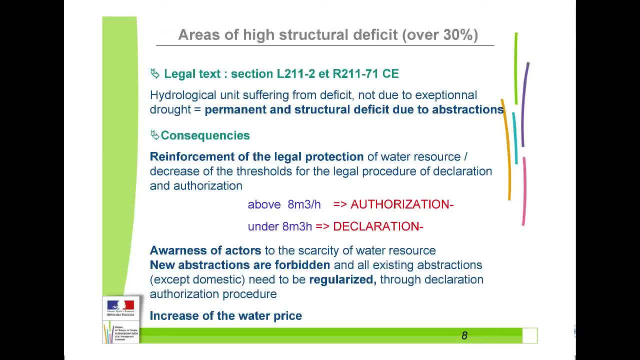 And all existing abstractions, except domestic, need to be regularized through declaration or authorization procedure, And no new abstractions are authorized. So new abstractions are forbidden. as soon as the water is released, The balance is not recovered. Another consequence is the increase of the price, but in another hand it allows to improve. 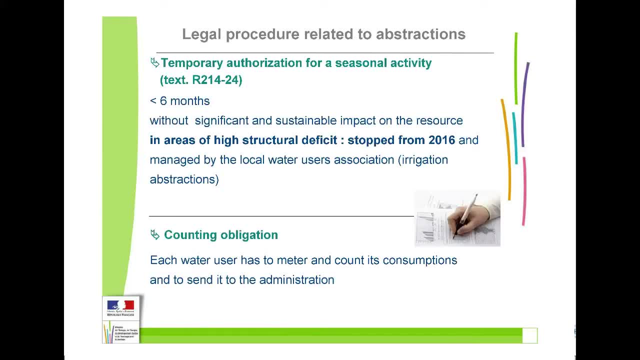 the funds dedicated to water saving actions. Then we have another tool, that's for temporary authorization, so shorter than six months, without significant and sustainable impact on the resource, But the thing is that It was very often used for abstractions that were permanent. 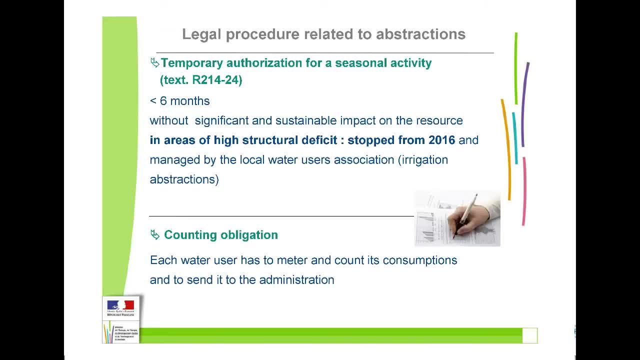 So in the areas with high structural deficit, the LAO asked us to stop this authorization and to be So. they are managed. they are included in local, So in collective irrigation and managed by a local water user as well. Thank you, Thank you. 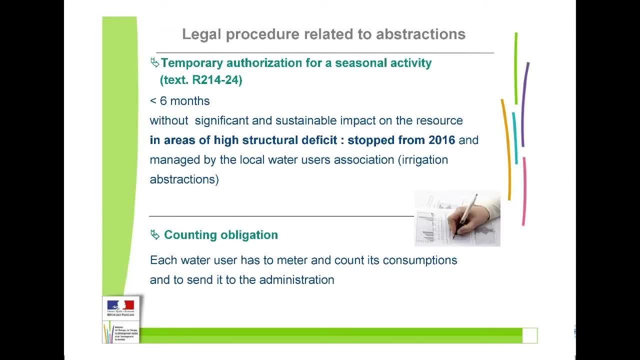 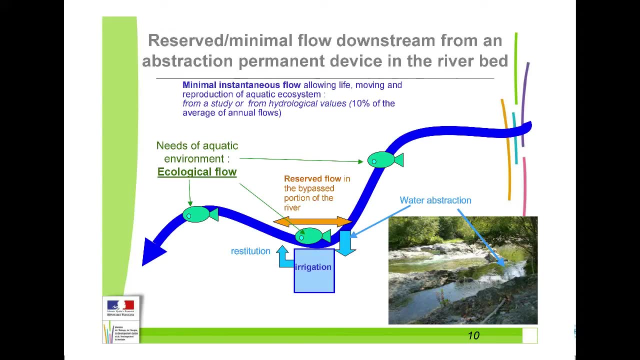 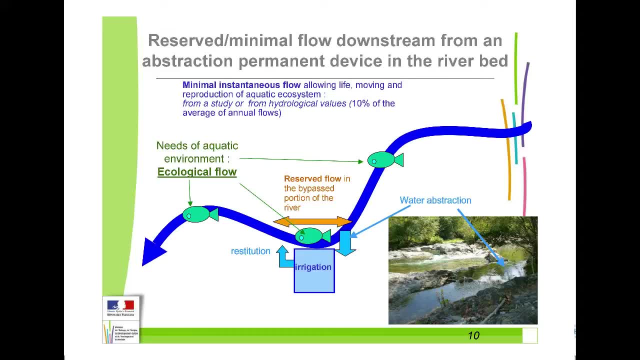 We have a lot of gravity irrigation in Languedoc-Poussin. The thing is that you have a bypass portion of the weaver, and so these tools ask to the users to let a minimal instantaneous flow, allowing life-moving and reproduction of aquatic ecosystems. 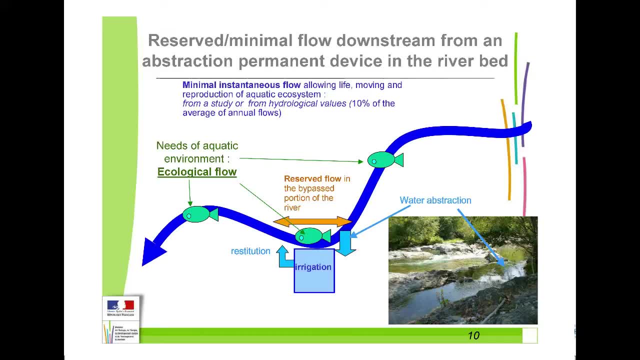 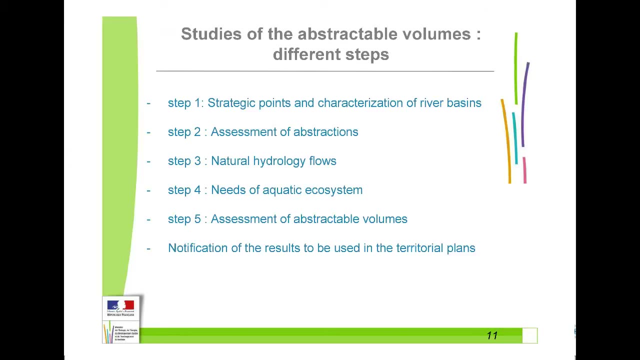 So the value comes either from a study or from hydrological values. So generally, in the general case, it's 10% of the average of annual flow. So then we have two. We have to implement these studies of abstractable volumes. 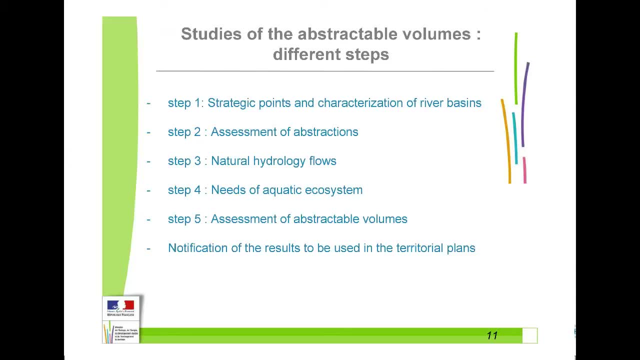 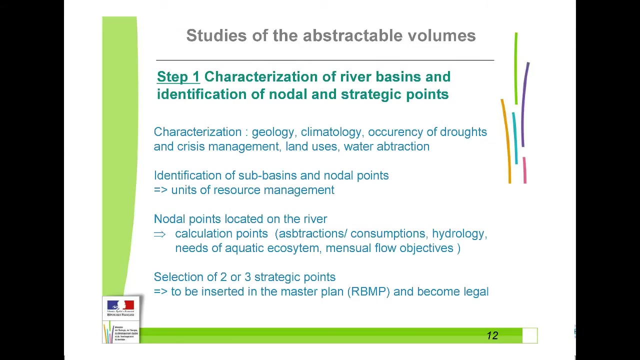 and so they have got several steps, so five steps. And then, after another step, John was by the administration to make a notification of the residue to be used in the territorial plant. So first step was a characterization of river bedding and identification of nodal and stratigraphic. 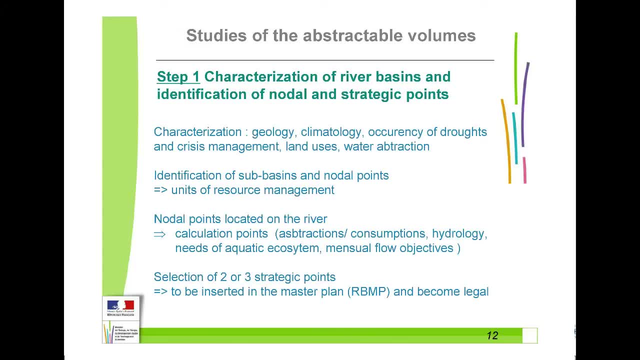 So characterization was done according to or using ecology, climatology, the currency of drugs and crisis management. the land uses the water abstraction. The objective of this first step was to identify sub-bassin and nodal plants, closing this sub-bassin on the weaver. that will be units of future resource management. 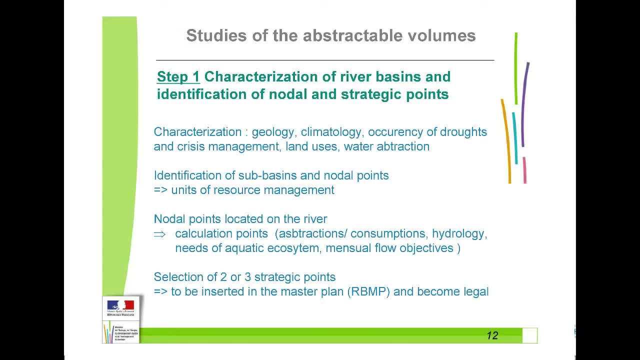 but also units on points of calculation. So we had generally maybe 10 or 15 points or sub-bassin for every river, But we couldn't have more because of course after studies would have been very long I have not said, but studies of abstractable volumes. 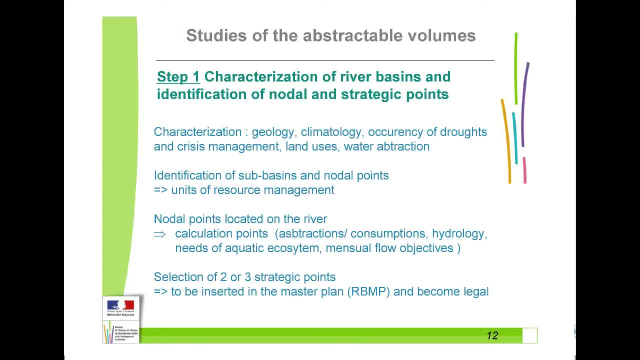 it takes about two years. so they are big studies. So, anyway, we had these nodal points and we had to make a selection of two or three of these points to become stratigraphic points. that means that they have been included in the next RBNP. 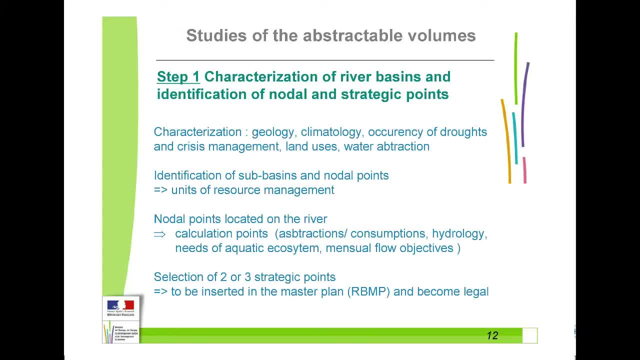 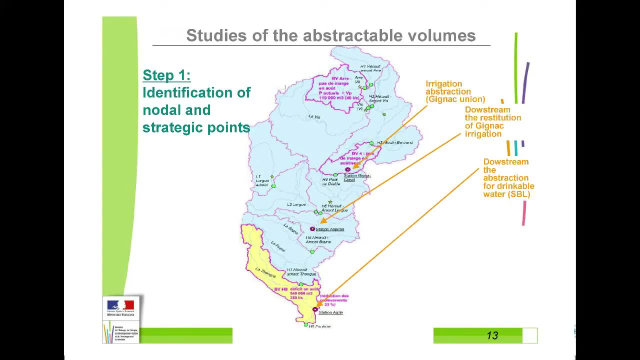 And the flow objective. you will see that we have flow, a monthly flow objective, So we have to be consistent with the flow objective. Eventually the funding will become legal, So we have to be effective. In this slide you can see an example. 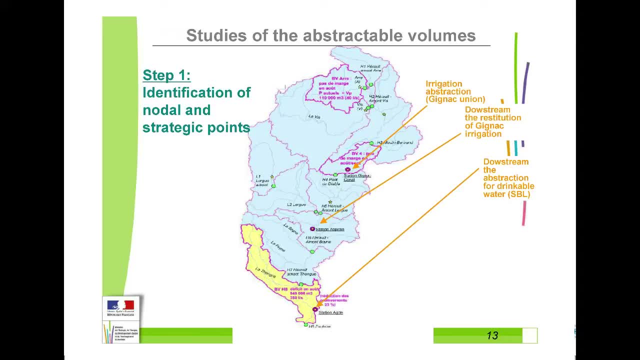 It's the Ihreux River. it's west of Montpellier. Here you have got the river and they have got afliens. You can see every different sub-bassin, The closing point, so nodal points, in red color and the stratigraphic point in purple color. 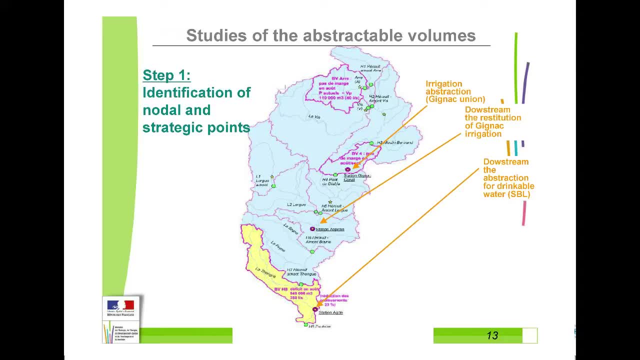 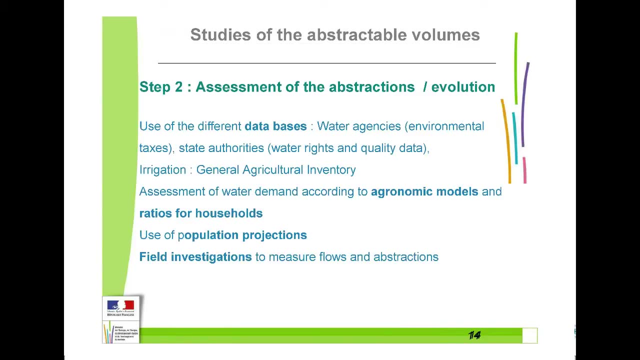 So this is the that were upstream and downstream, big irrigation, abstraction and the closing point of the river basin not far from Arcta. So a certain part of the study was the assessment of abstraction. So we used different databases from water agency, from state authorities, water rights quality data and so on. 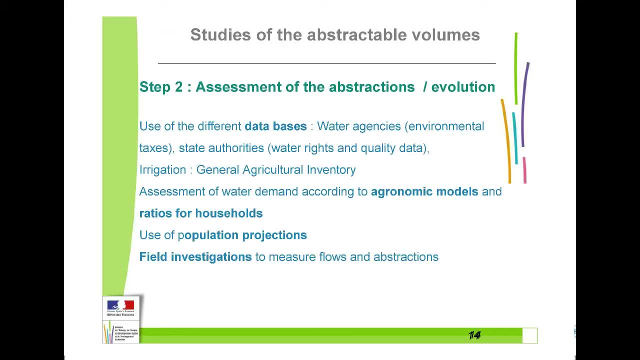 Irrigation, general agricultural inventory was used and also, in some cases, we used agronomic models to assess the demand and ratio for household use of population projection and, moreover, field investigation to measure flow and abstraction. So, especially with irrigation- gravity irrigation- it was important to measure flow. 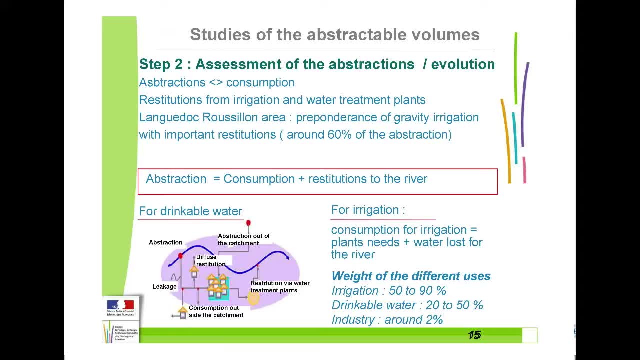 The same thing. The same thing is that we made the difference between abstraction and constriction because we have a lot of restitution to the river, either from irrigation use- especially when it's gravity irrigation- or from water treatment plants. That means that reuse for us can be a solution, but if we are very downstream of the river basin, 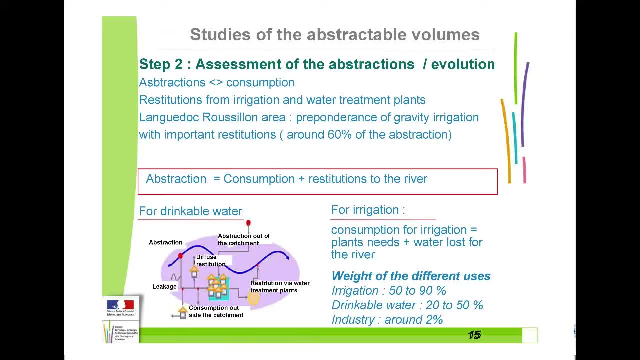 Otherwise we consider that we The restitution gives some flows to the river that is useful. So this step allowed to improve knowledge, of course, and to know the weight of the different uses In our area. we have about Irrigation is a big abstraction: around 50 or 90% of all irrigation uses in our area. 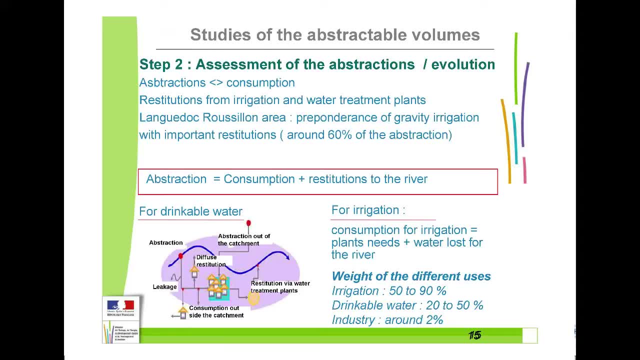 of all attractions, depending on the river, And whereas drinking water is about 20 to 50%. Even if we have a lot of tourism during the summer, the industry is very low, around 2%. But you will see that in the territorial plans. 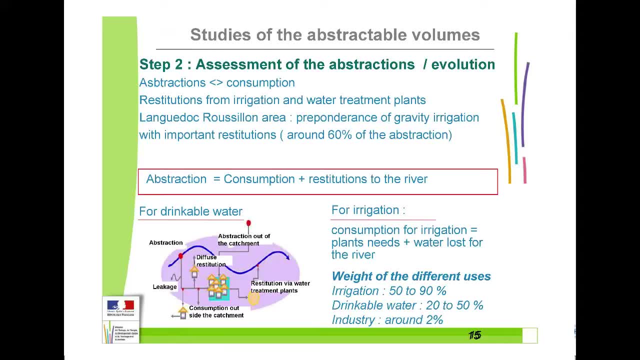 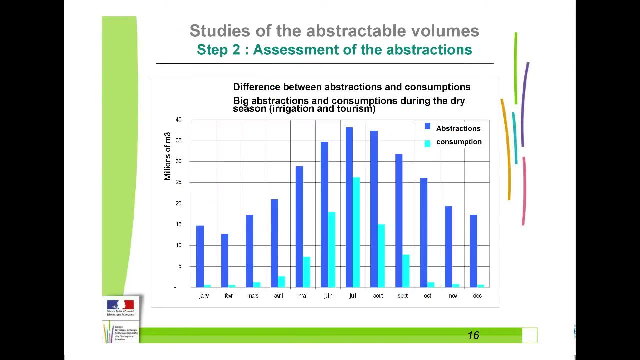 all the users, all the stakeholders have to be involved so that water management could be a success. Another result was this kind of graph where you can see the monthly value for the year And first we can see the big difference between abstractions in blue and construction in this other blue. 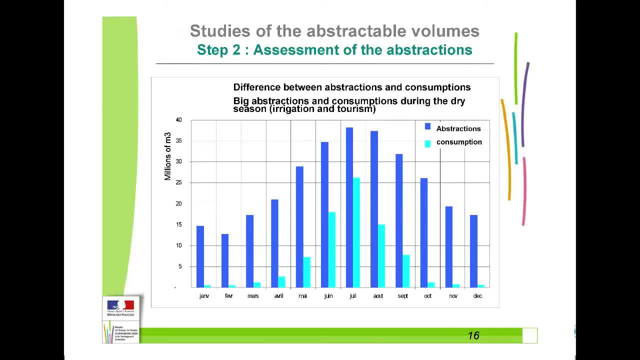 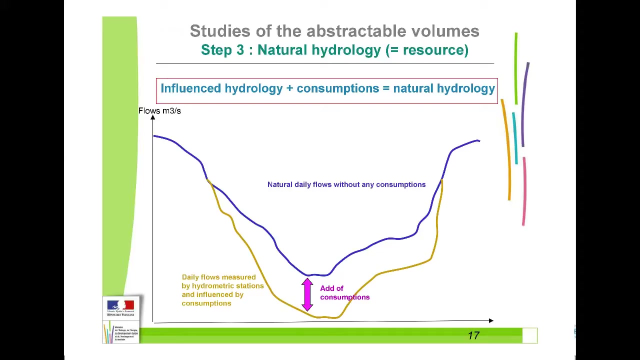 And then we can see that big abstraction are done in summer or in spring And unfortunately it's the season where natural flow are low. So this is really the months where we have to face to challenge the water management. Then, as a step three, we had to assess natural hydrology. 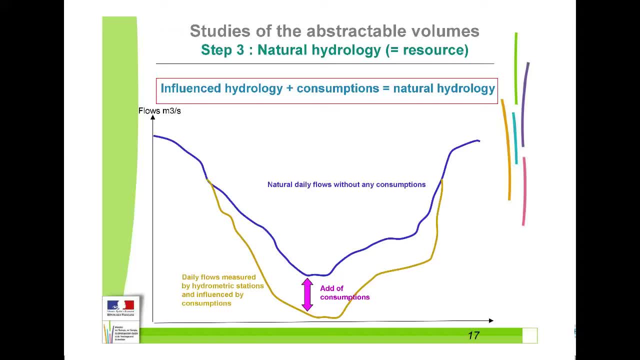 with this very simple equation. In this example you can see daily flows. so in yellow so daily flow measure from hydrometric station and influence by construction. But if we hadn't any construction then we should have this flow in the curve in blue. 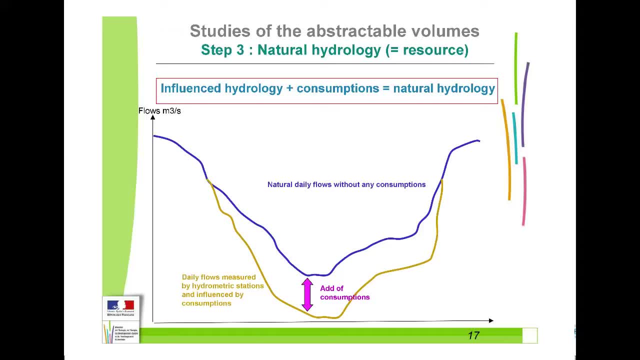 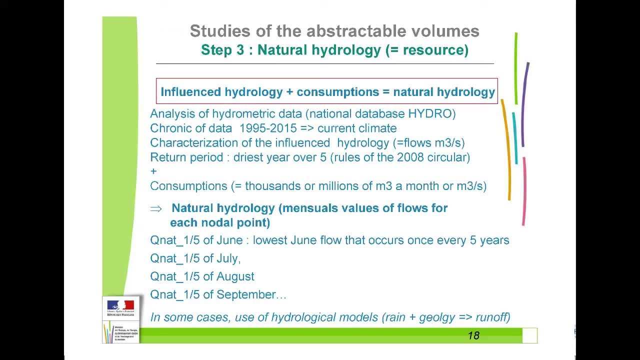 So to get that we add construction to the chronic of influence flows, We have done the analysis of hydrometric data from the National Database Hydro and with the use of chronic data, but not too old data, not too old years, because we wanted to use the current climate. 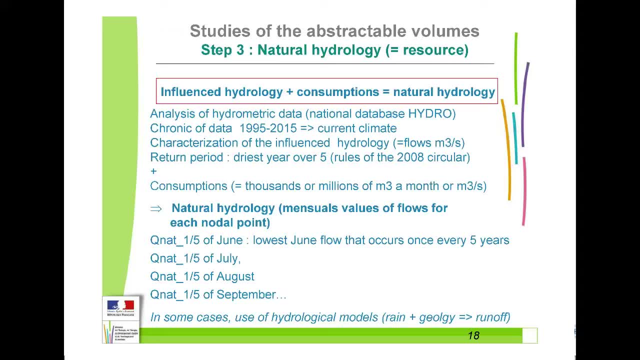 because climate is changing, And then it allowed to make the characterization of influence flow And we applied for statistical action. We applied the return period of the- what we call the driest year over five years to be okay with the rules of the 2008 circular. 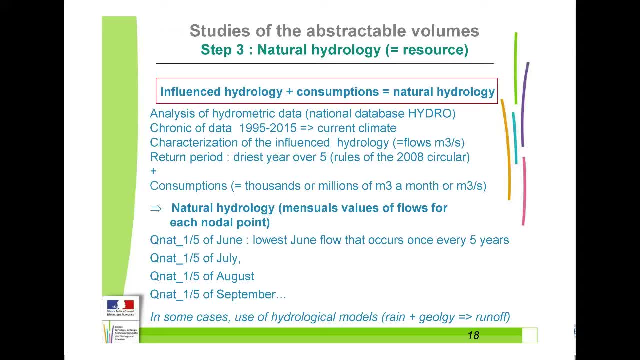 and with the main strategy. Then we had the construction and we get the natural hydrology, So, for example, so for every month, for example in June. so this value was used after to assess the abstracted volumes, And so it's the lowest June flows. 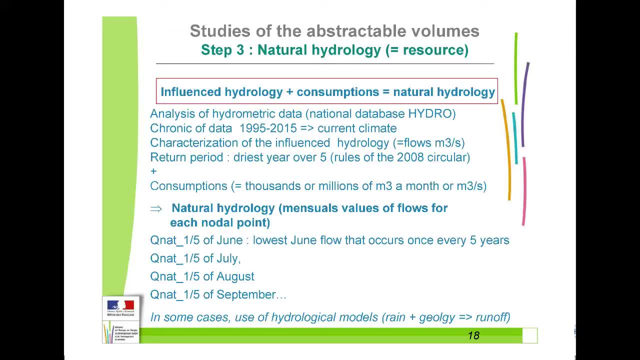 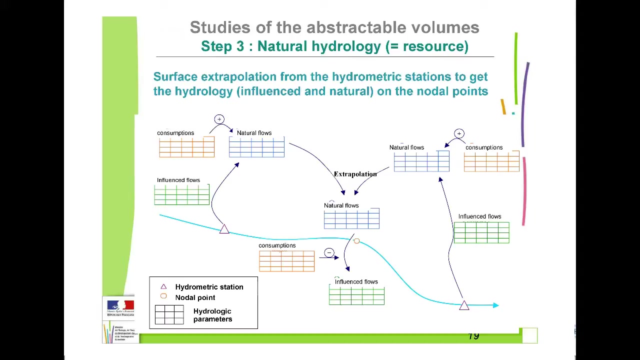 that occurs once every five years. In some case, when we had very few hydrometric data, we had to use hydrological modeling, So using rain data geology to assess the flow through and runoff, And after, when we didn't have any hydrometric station. 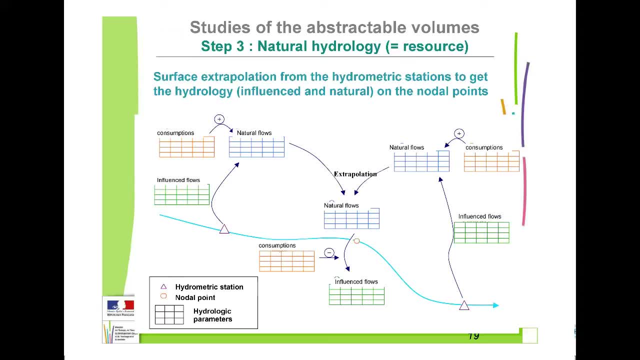 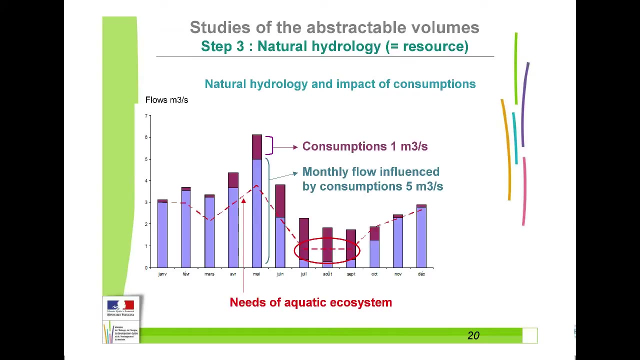 for some nodal points we had to apply extrapolation from the surface of the river basin. So you can see that for each hydrometric station we had- and we had influence flows through the construction to get natural flows. So then we get this result. 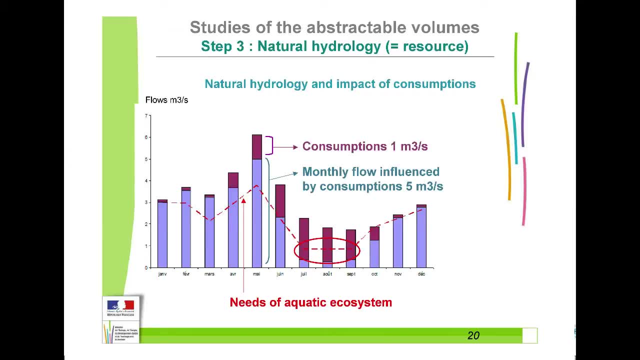 This example you can see, so you have. for example, in May in this basin we have about six meter cube for the natural hydrology and one meter cube for construction and so five for influence flow. And you can see in the red color. 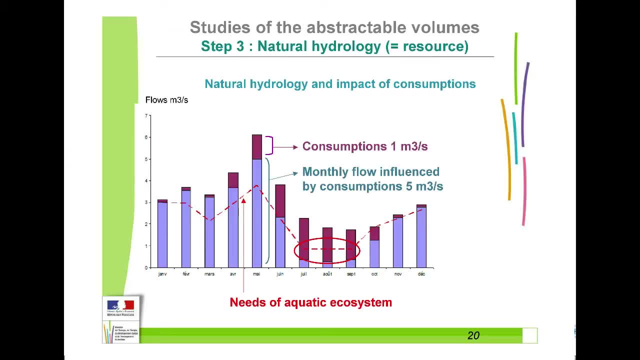 it's the curve of the needs of aquatic ecosystem. You can see that in July, August and September, because of the construction, the influence flow are very low, about less than one cubic meter, And that's to say that we are not in structural deficit. 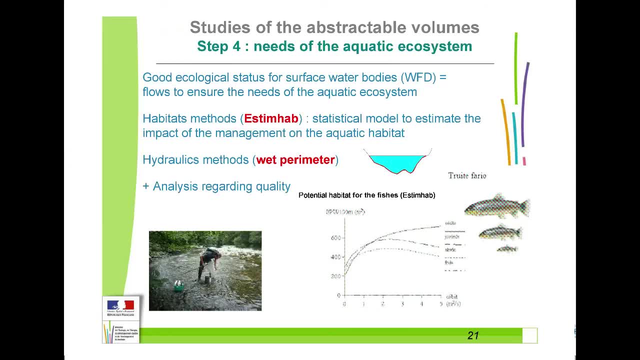 So how this needs of aquatic ecosystem were assessed. that was the first step. So good ecological status for surface water bodies is a requirement of the Water From Water Directive, And that's to say that we had to assess the flow to ensure the needs of aquatic ecosystem. 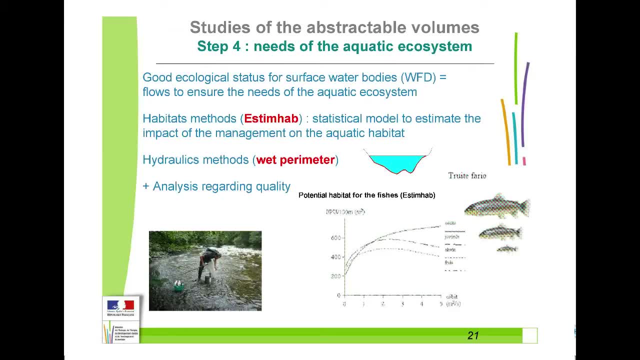 For that we use the method, the model called STMAP, That's to say that it estimates the impact of the management of the aquatic habitat on the aquatic habitat. In this example you can see that if we decrease the flows then we decrease the potential habitat. 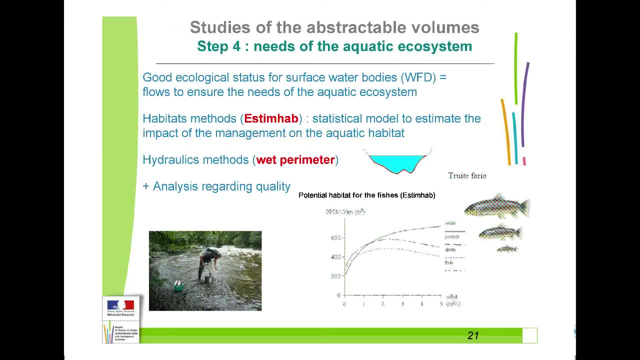 for the fishes which are identified in this portion of the river, in this portion not far from the normal point, And so experts help us to identify the flow, the ecological need for ecosystem. Moreover, we use quality data to improve the analysis. 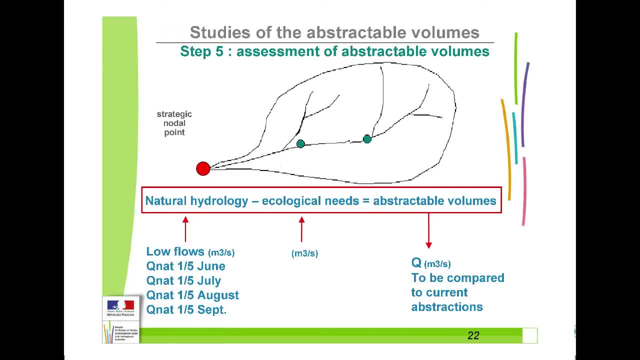 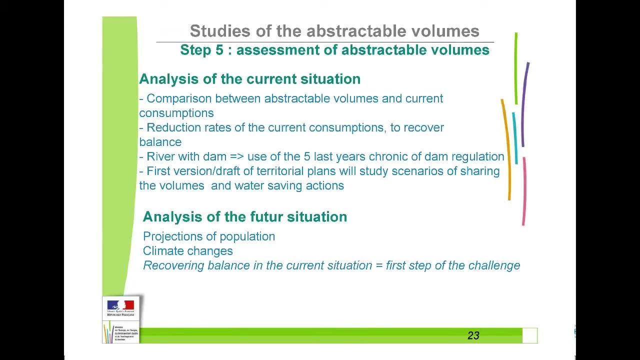 Then, as a step five, we had all the data we use we wanted, and then we could make the difference between natural hydrology and ecological needs to get the abstractable volumes. Then we could make the comparison between abstractable volumes and current consumption. 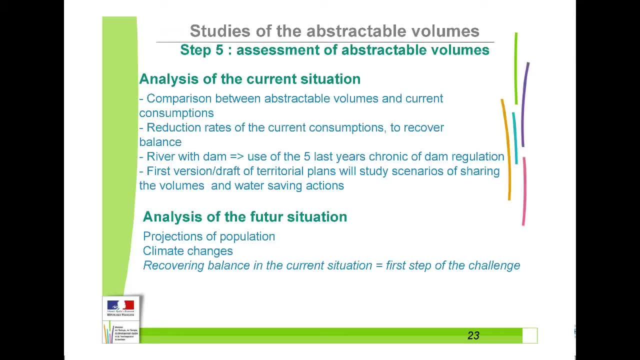 We could identify the different sea basin reduction rates for the current consummation. to recover the balance In the case of river with dam, then we had to use the five last years chronic of dam regulation to add that over the natural hydrology. And then in this step, 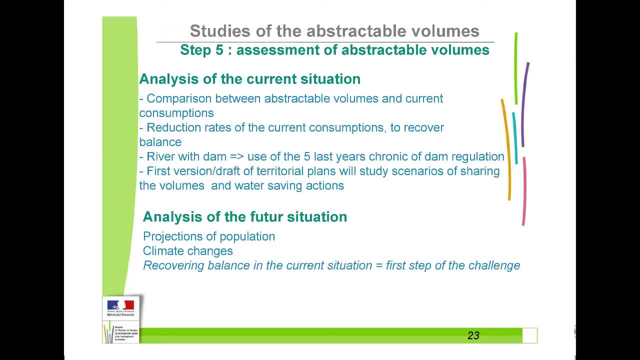 we in some case we had the translation and draft of territorial plans with some studies of sharing volumes and water saving action. But the thing is that first the analysis of the current situation and the recovering the balance in the current situation is often a really challenge. 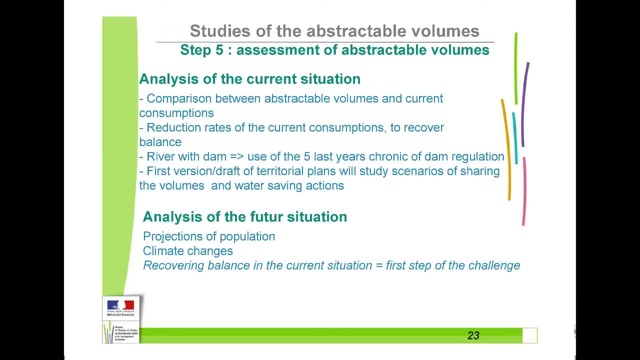 because the rate of reduction consumption are very high. Anyway, we had in some case projection of population and of climate changes, But the thing is that if we were in the current situation, if we do action of saving water and recover the balance, it would help us. 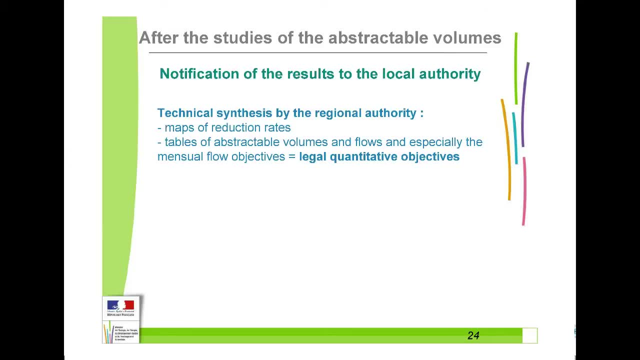 to adapt to the climate change. Then, after these studies, we had to make the notification of the results to the local authority so that it could be used for the territorial plans. So what does it include? It included. so one later, but with: 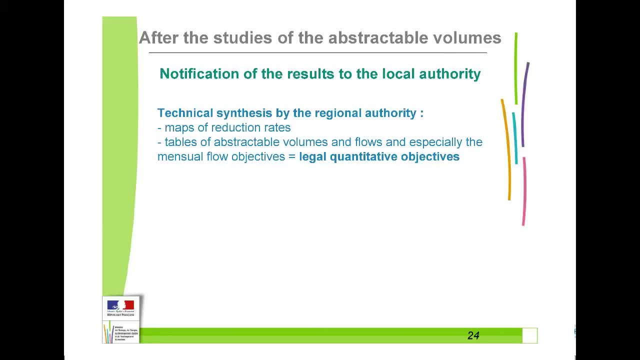 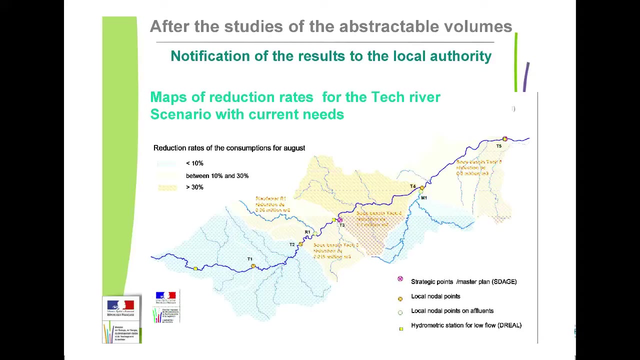 so maps of reduction rates and with tables of abstraction volumes and flows, and especially the monthly flow objective. that are our legal quantitative objectives. Here is an example of a map. You can see the blue part when, where it's okay, we are not far from the balance. 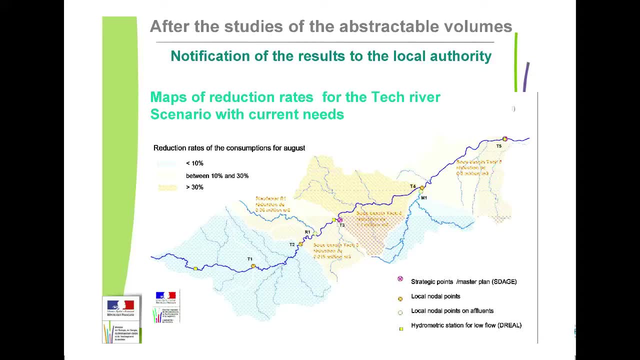 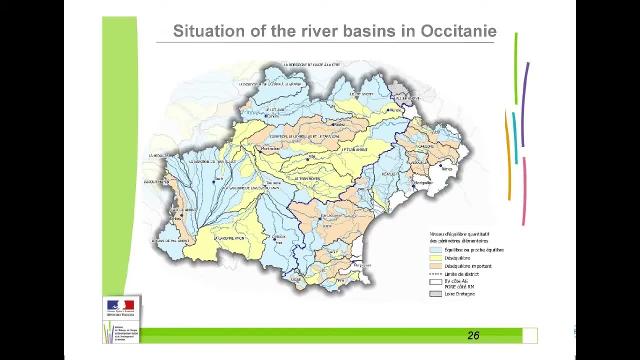 And in the yellow part when so the rate of reduction are between 10 and 30%, And in orange it shows the area of high deficit. This is the situation in whole Occitanie region, So with two parts, one included in the river district. 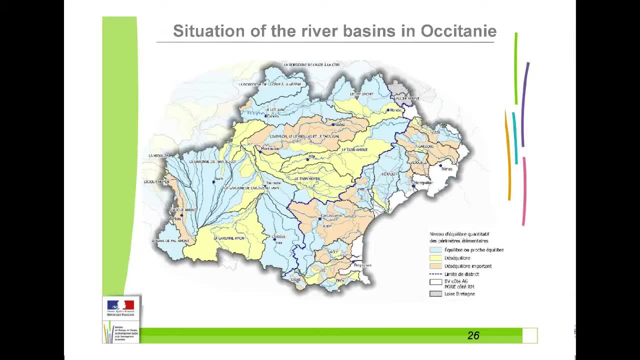 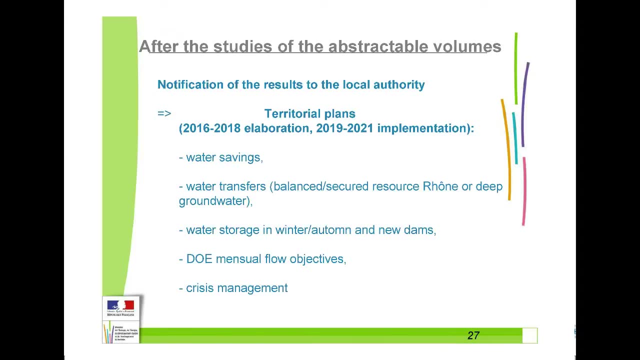 in the district of the Mediterranean and the other part in the district of Hadrocaron. So after the studies. so we- I spoke about the notification of the results- and also, yes, we had to first make the elaboration of this territorial plans. 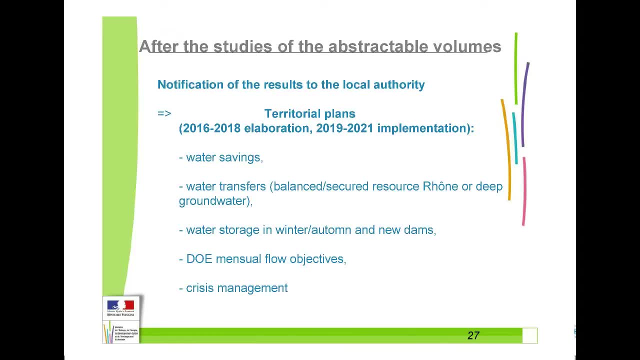 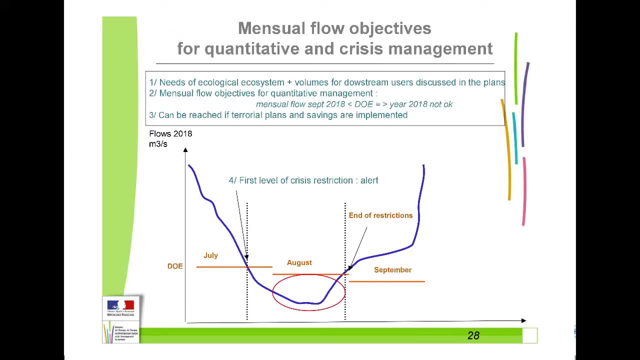 then the implementation, So water saving, water storage and crisis management and the monthly flow objective. Just a word, a few comments about the monthly flow objective. So first it is finally the needs of ecological ecosystem And, if we are not downstream, the river basin. 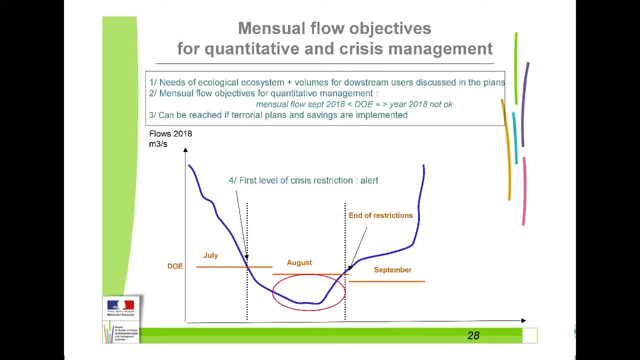 then you can add volumes for users that are downstream. And then, secondly, it's used to assess the balance. That to say that, for example, in fact it's not same term, it is not September, but it's August In this example. 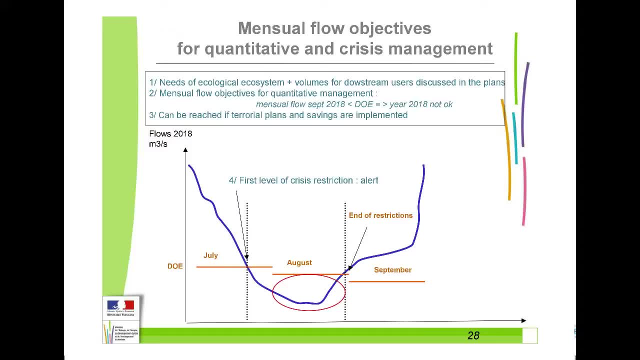 you can see that we have three monthly values for this flow objective, So July, August and September, And here it was the two 2080 year, And you can see that in July we begin to have flow under this objective, So that to say that we 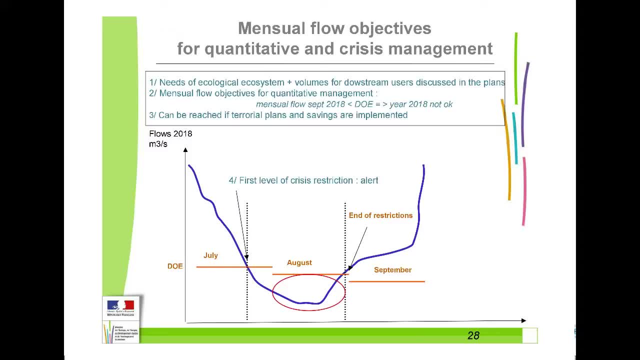 we entered in the first level of crisis restrictions, or in ALERP. So and you can see that in August flow are very, very low and under the objective. So after once the year is completed, when we have to make this assessment, 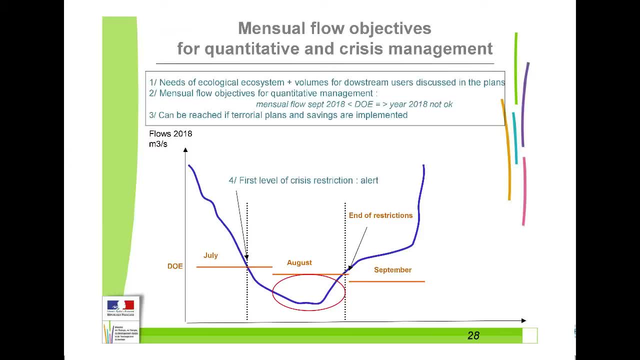 for this year and for this point, we consider that the average flow of August was under the objective and so that the year of 2018 won't be okay for the water, the constitutive water manner, And we'll do that for a chronic of five or ten. 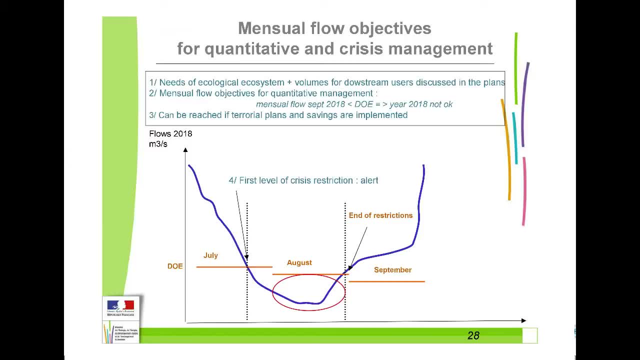 ten years and to check if the rule of the circular 2008 is respect, That to say, just one year, not okay, and the use of crisis management over five or two, over ten. So the thing, the third point, is that we do. 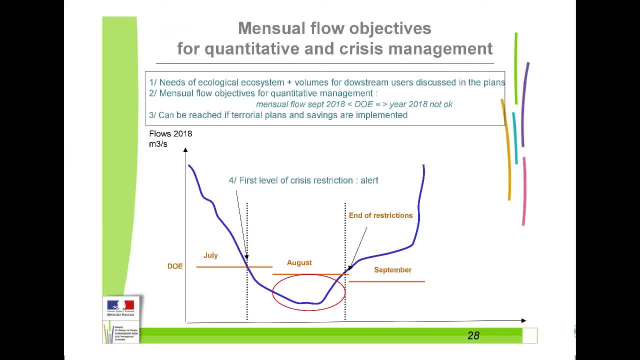 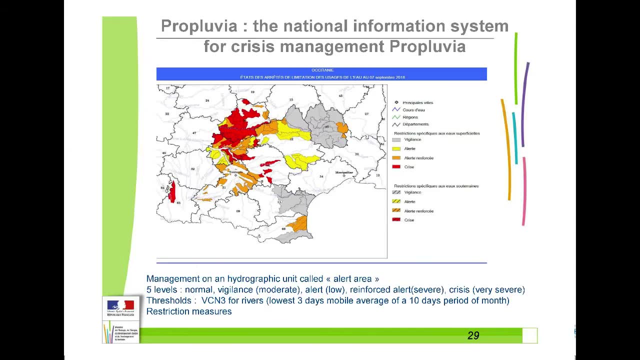 we cannot reach this objective is if territorial plans and saving actions are not implemented. So that's the first action. It's very important. Just a slide to present you a a crisis management. So we do that in France. through, we have got. 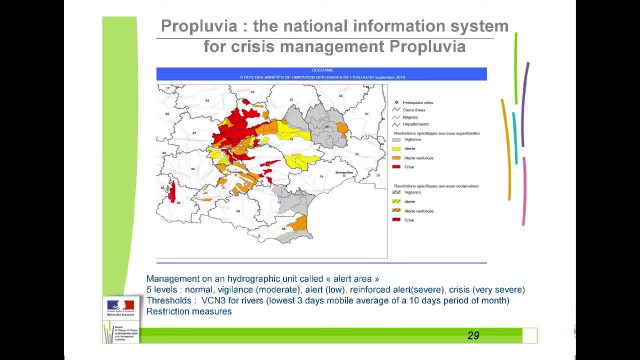 management plan on the scale, on the department scale, If river is in some case, we have got rivers within two departments, So we have. so the management plan will manage that through and will be so developed during between this different department. 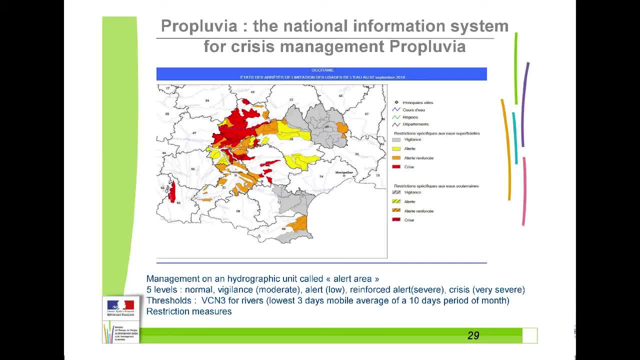 We are using so hydrographic unit called alert IR and we can. we have five levels, So normal, vigilance, alert, reinforced alerts and crisis, And for all this level we have restriction measure We are using so you. 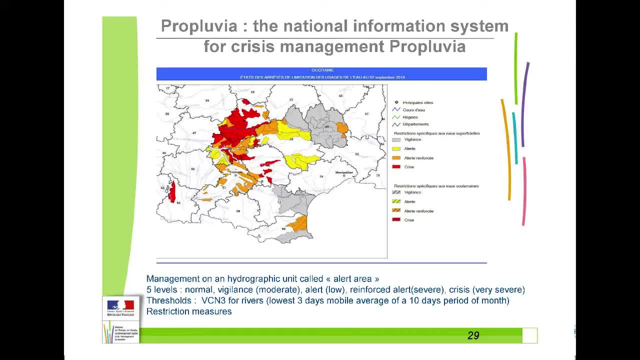 so now we are using the flow menstrual flow objective, as I just told you in the former slide, And also other indicators that are. so that's the lowest three days mobile average of 10 days carrier And we have an information system. but 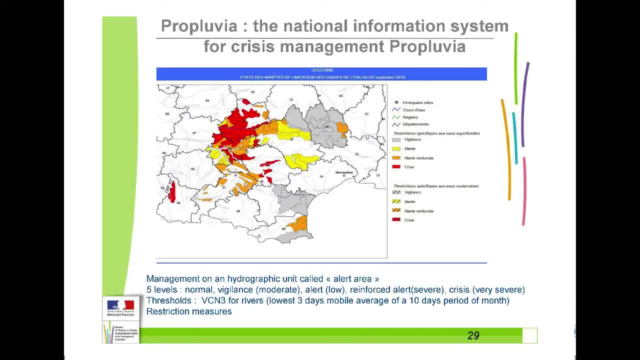 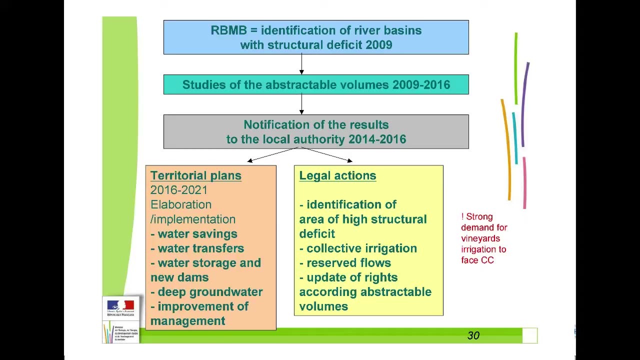 because if we want the actor to respect restriction, they have to be able to get the information very quickly. So just this last slide to summarize the approach and the strategy. so we had the identification from the available data of river basin with the structural deficits. 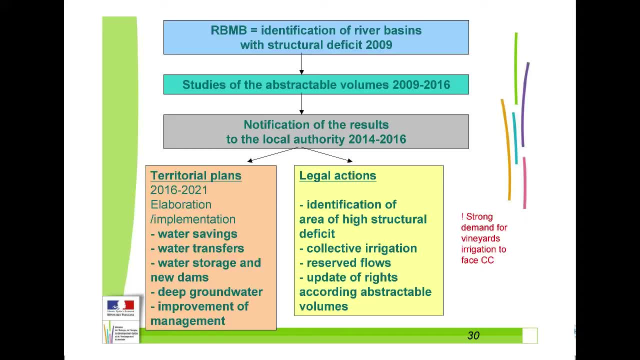 That was done in 2009.. Then we had the studies of abstractable volumes between 2009 and 2007.. Then we had the notification of official later of the result to the local authority should be used in the elaboration for us then in the implementation. 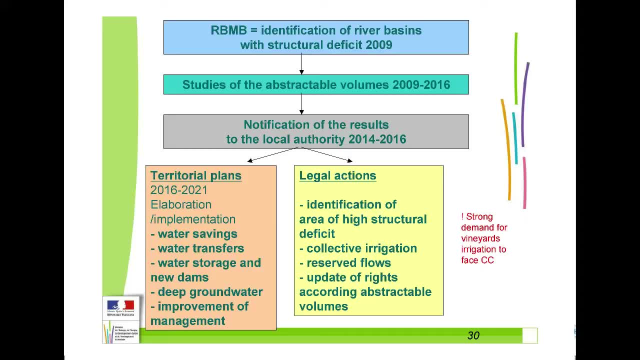 of terrorism of the project. And then we have the legal action to follow the territorial plans with the different action, So water saving, water transfer, water storage, groundwater management and improve of the crisis management. And then we have also legal action.